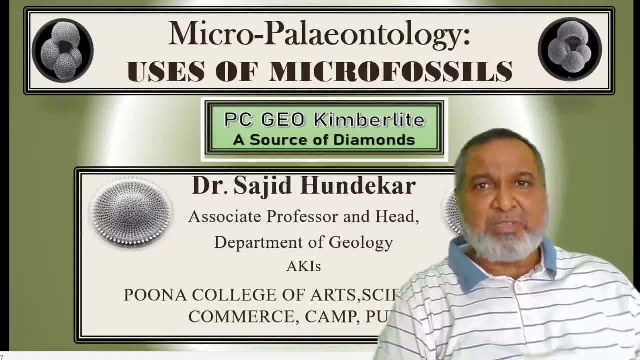 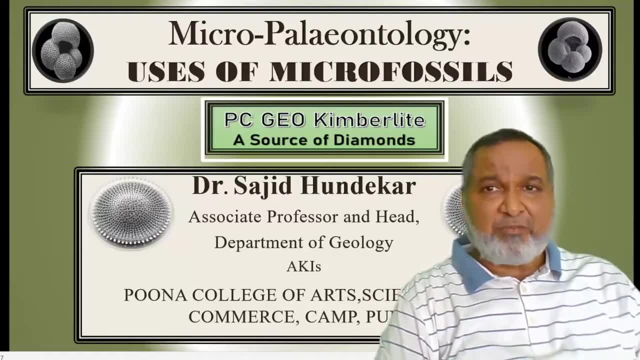 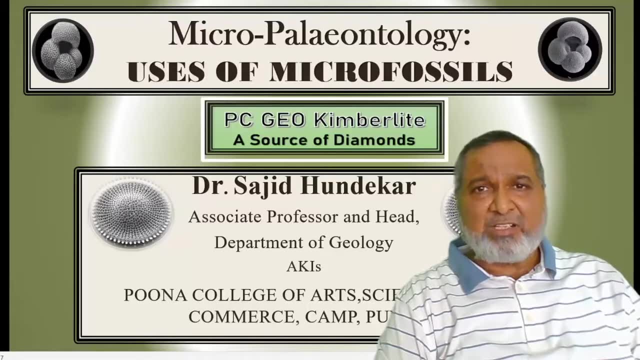 Hello viewers, welcome to my channel, PC Geo Timberlite. Today we are going to see another topic from micropanetology: the uses of microfossils. I am Dr Sajid Undekar, Associate Professor in Head Department of Geology, aka Spinoff College of Arts, Science and Commerce CAMP. 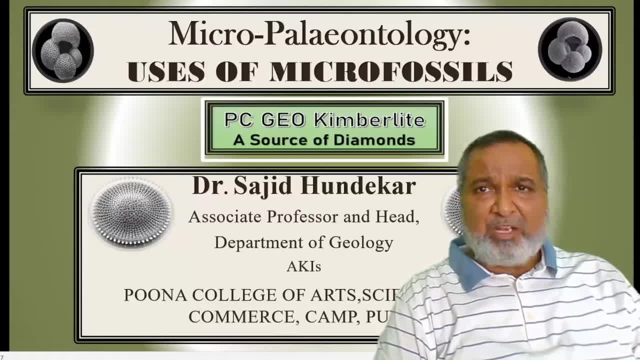 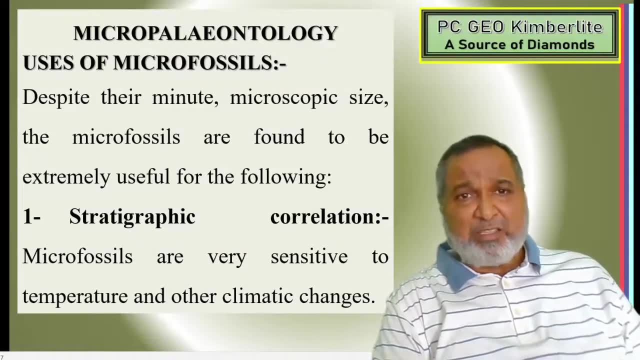 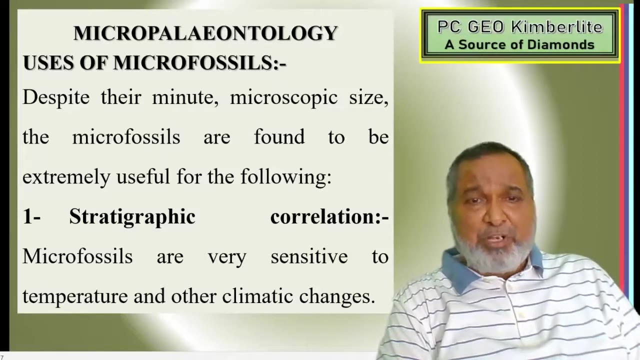 Pune, Maharashtra, India, Affiliated to Savitribai Phule University, SPPU, formerly known as University of Pune. The uses of microfossils: Despite their minute and microscopic size, the microfossils are found to be extremely useful for the following. The first, important. 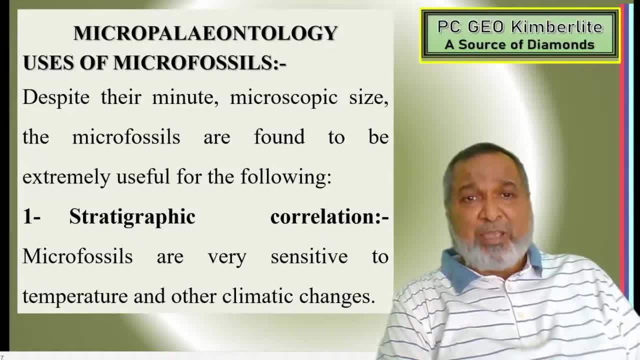 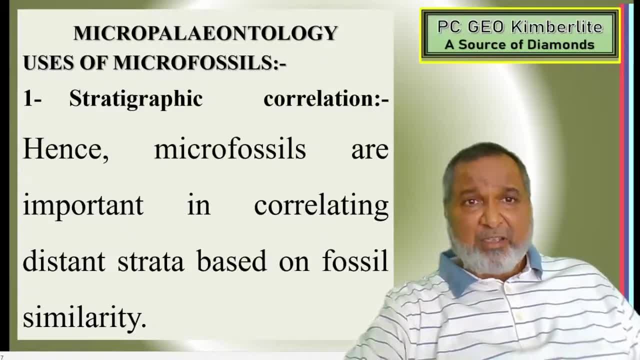 use in stratigraphic correlation. Microfossils are very sensitive to the temperature and other climatic changes, So with this, hence, the microfossils are important. In the case of microfossils, they are very sensitive to the temperature and other climatic. 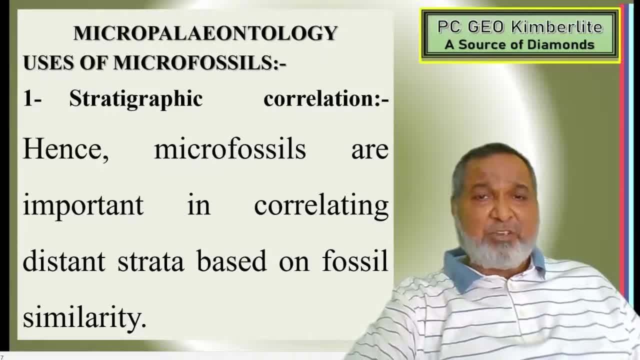 changes. So the microfossils are very sensitive to the temperature and other climatic changes. They are used for biostatic group. They are used to correlate the distance strata based on the fossil similarities, Microfossils, especially poles, spores and under-foray manifolds. 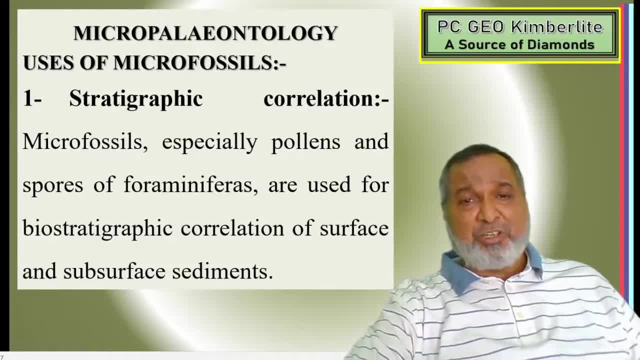 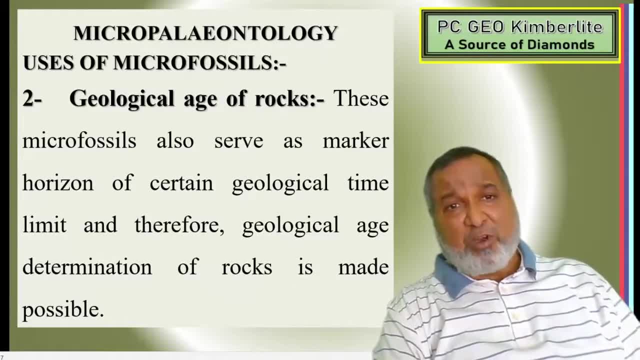 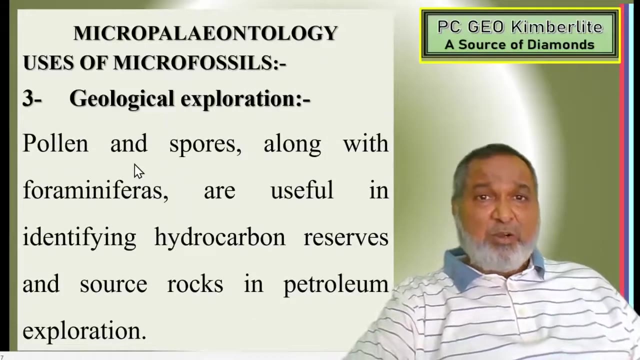 are used for biostatic group correlation for surface and under surface sediments. The second important one: geological age of rock. These microfossils also serve as a marker horizon of certain geological time living and therefore geological age determining the of rock is made possible. Third one: geological exploration. Pollens and spores, along with 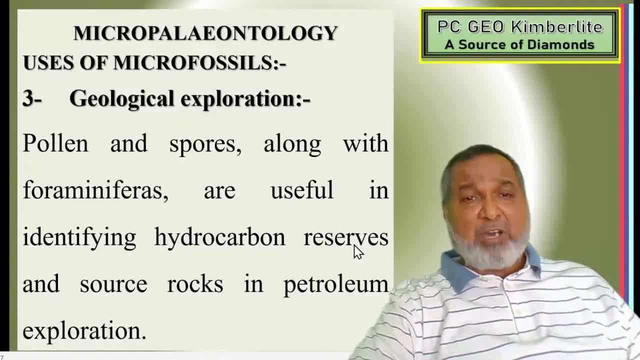 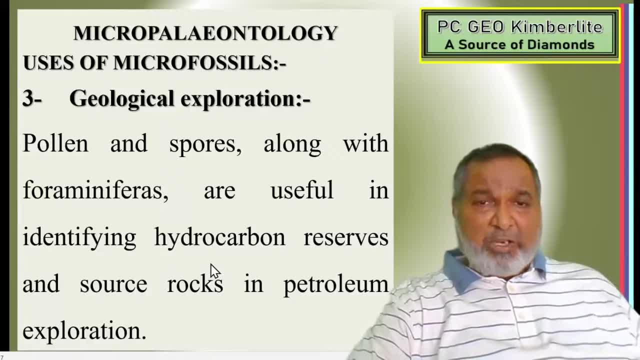 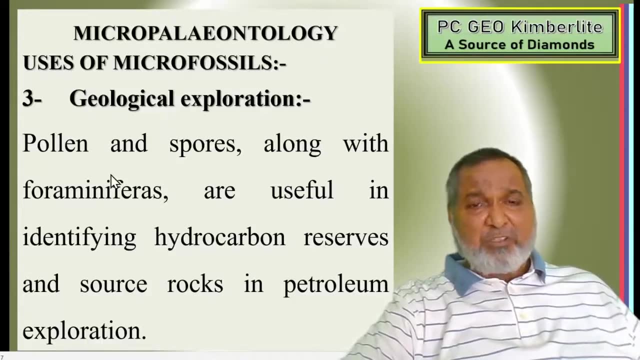 water minerals are useful in identifying hydrocarbon reserves. that is, the petroleum oil and natural gas, the source rock in petroleum exploration. So 90% of the oil and natural gas is coming from the tertiary. So we have been looking for water and refills or pollens or spores. 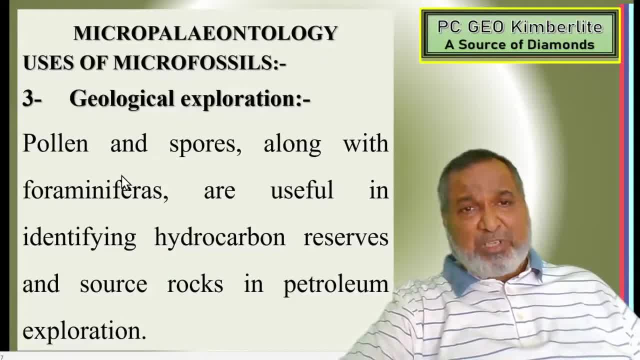 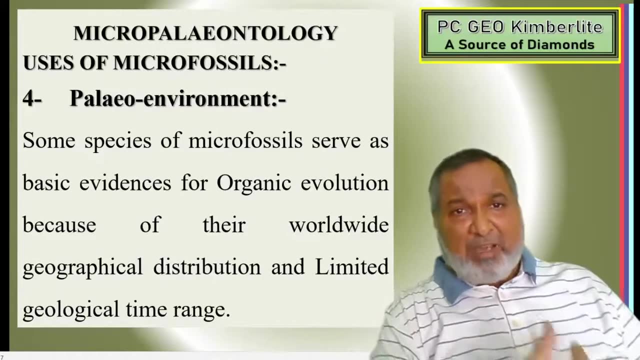 from the tertiary. So India is trying to scan for those tertiary rocks where we can find out the pollens or spores, or for a many para, because these are the important raw material for the formation of oil and natural gas. The paleo environment to identify this important. 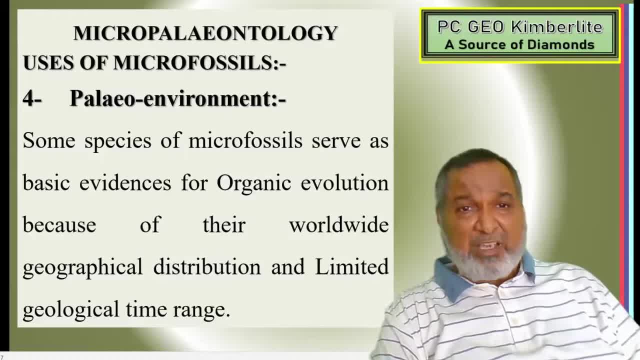 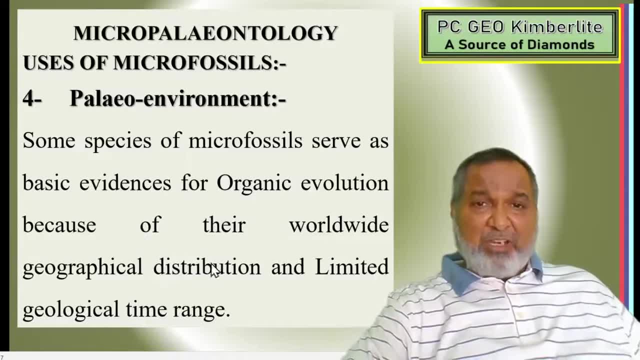 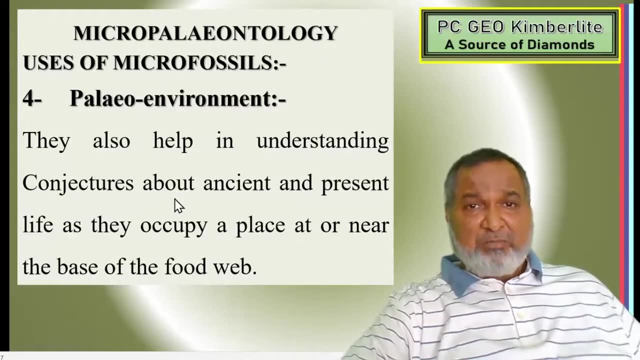 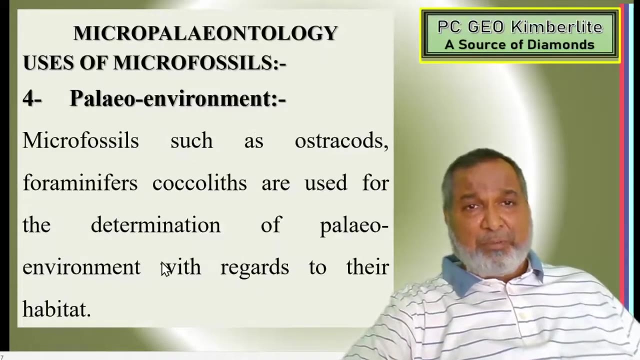 use of the microposal. Some species of the microposal serve as basic evidences for organic evolution because of their worldwide geographic distribution and limited geological time range. They also help in understanding conjecture about ancient and present life as they occupy a place at or near the base of food. web Microposals. 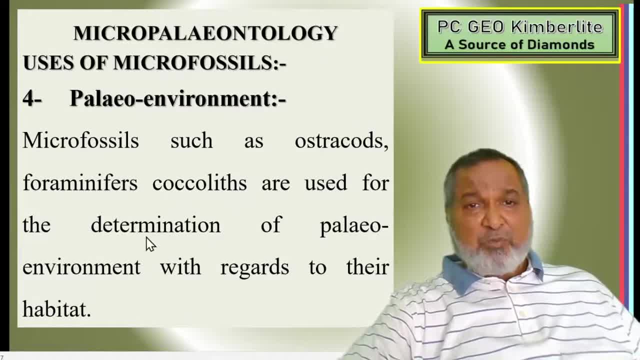 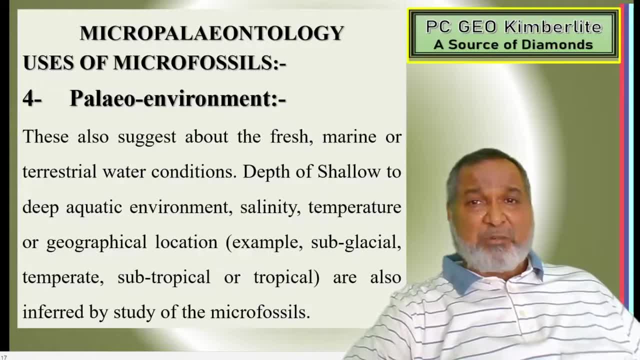 such as austro quartz foraminifera cocolith, are used for determination of paleoenvironment with regard to their habitat. These are also suggest about the fresh marine terrestrial water condition, Depth of shallow to deep aquatic environment, salinity, temperature or geographical locations. 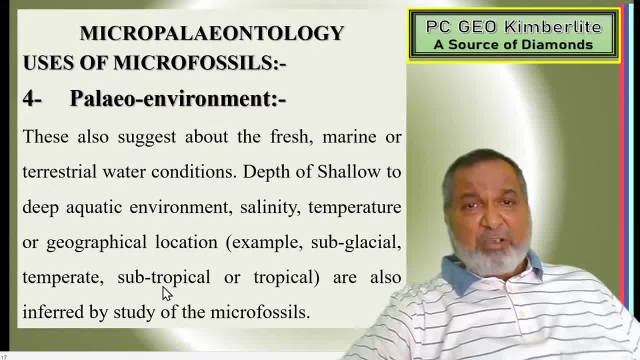 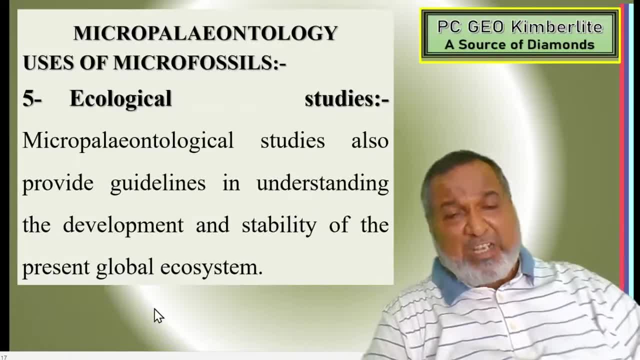 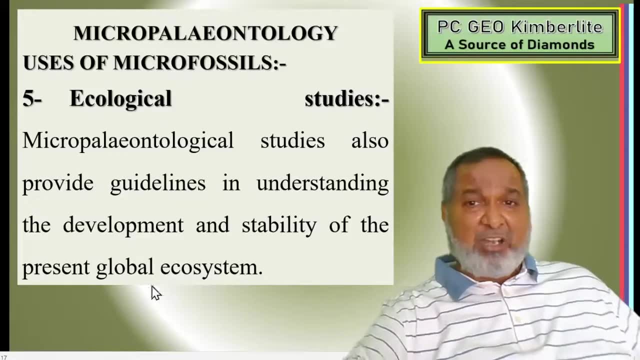 example, subglacial, temperate, subtropical or tropical, are also interfered by the study of the microfossils. Ecological studies, Micropedagogical studies also provide a guidelines in understanding the development and stability of the present global ecosystem. Important. 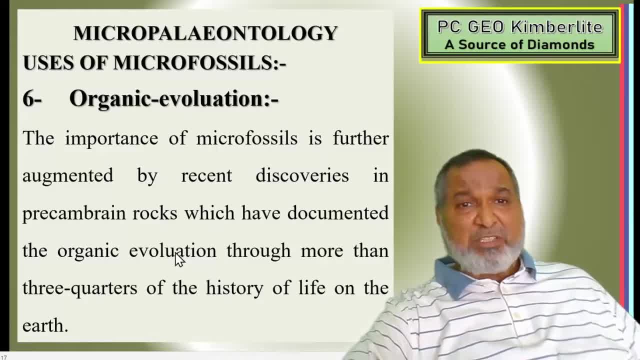 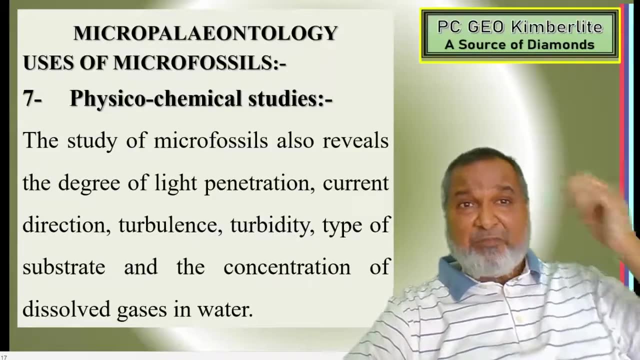 to understand these studies are the following: In this section we will cover the most important discoveries in the pre-cambrian rock ecosystem – the呀an, the Yin, the Yin, the ƒn and the ƒg fusion. 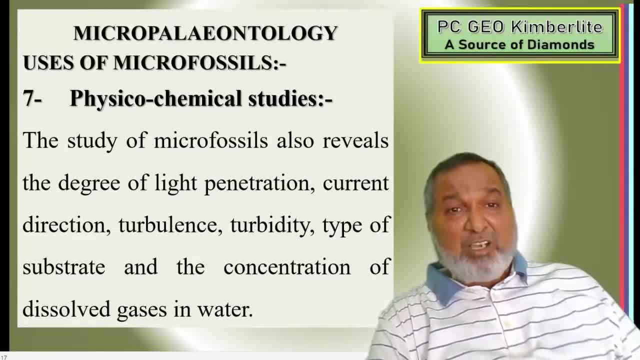 The importance of microfossils is further augmented by recent discoveries in the pre-cambrian rocks, which are documented their organic evolution through more than three quarters of the history of life on the Earth. Physiochemical studies, The studies of the microfossils also reveal the degree of light. 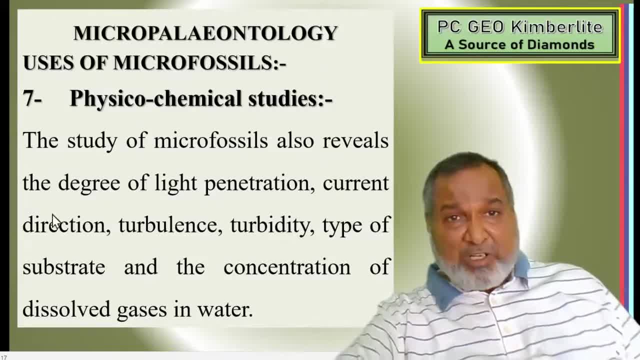 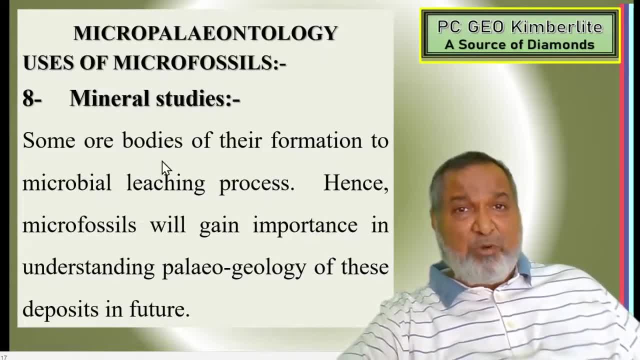 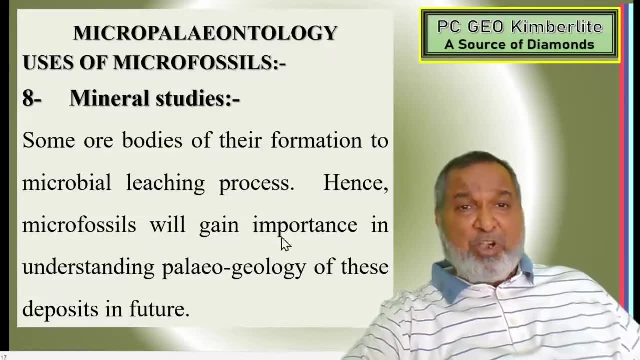 And the concentration of dissolved gases in the water. That will be going to useful to find out physiochemical studies, Mineral studies, Some ore bodies of their formation to microbial leaching process- Hence the microfossil will gain importance in understanding paleogeology of these deposits in nature. 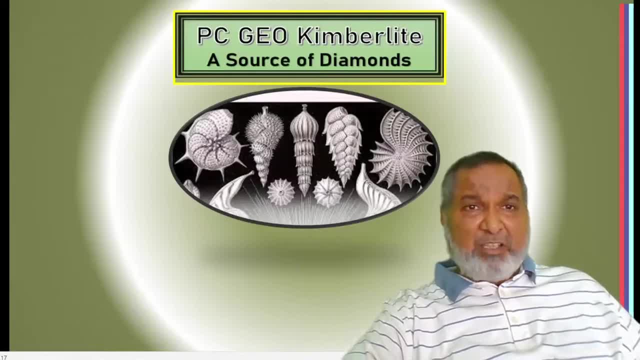 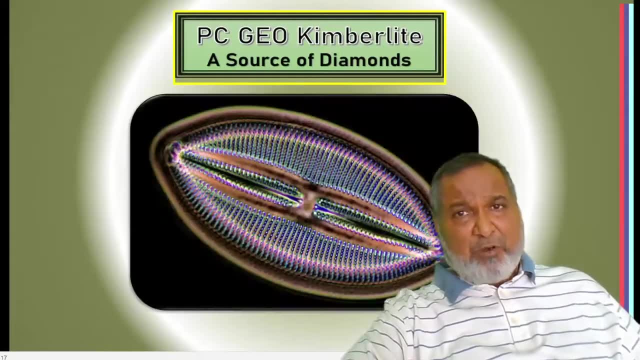 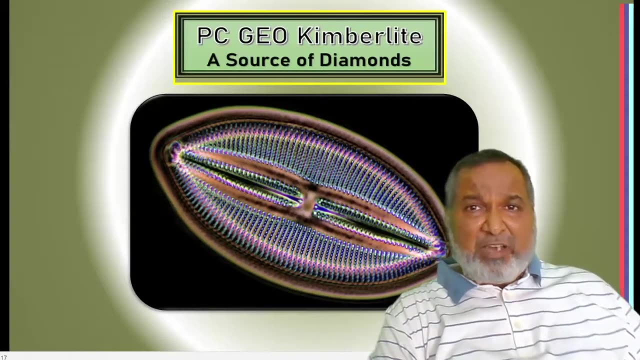 I hope this will be clear The topic, what we have done And the uses of the microfossils. Visit my website, pcgeochemberlitecom, For all whatever the videos are uploaded related to geology and scholarship. Thank you, Have a nice day.